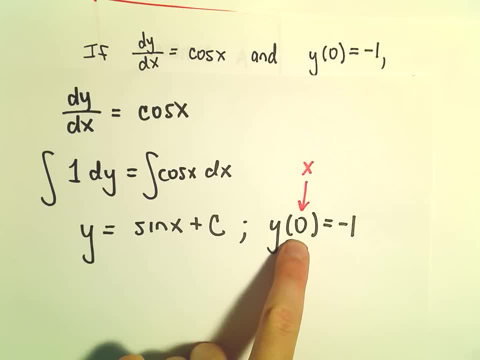 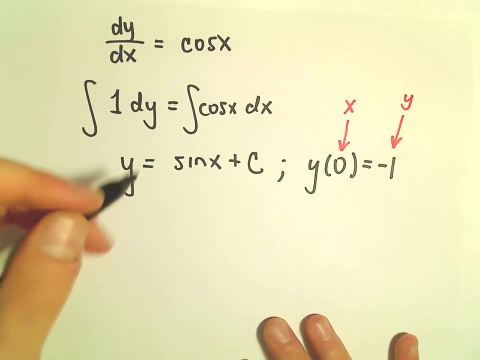 know used to bother me. So again, the stuff next to the y that represents your x value, The stuff you're getting out obviously was going to represent the y value. I don't know, I used to always want to plug this in for y, So be careful about that. Maybe you're. 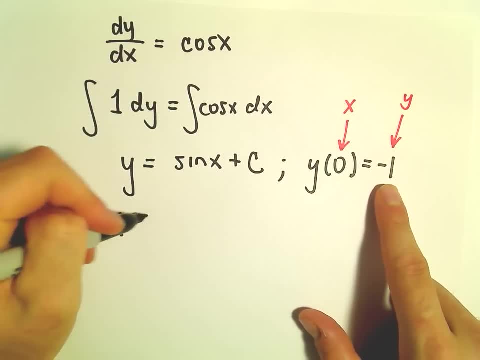 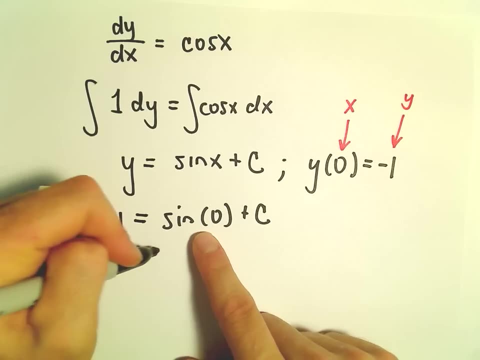 not as good as I am. So our y value is going to be negative 1.. We'll get sine of 0. Sine of 0 is 0. So we're left with our c value of negative 1.. So therefore, we would take: 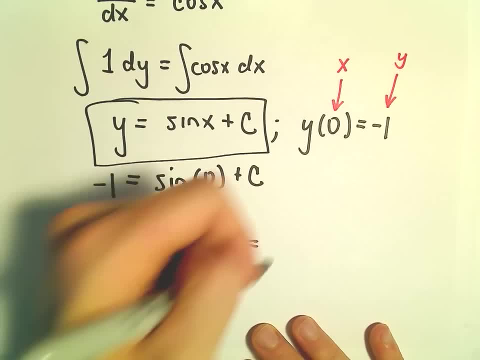 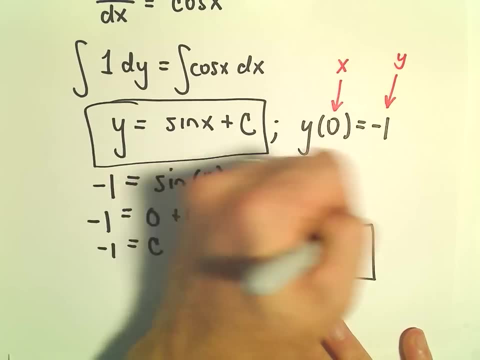 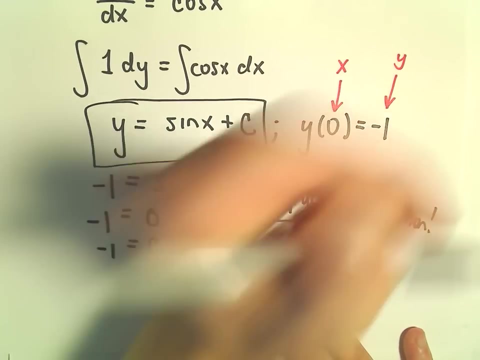 our general solution And our particular solution would be: y equals sine x plus c, which is going to be negative 1. And now we've got our particular solution, Thank you. 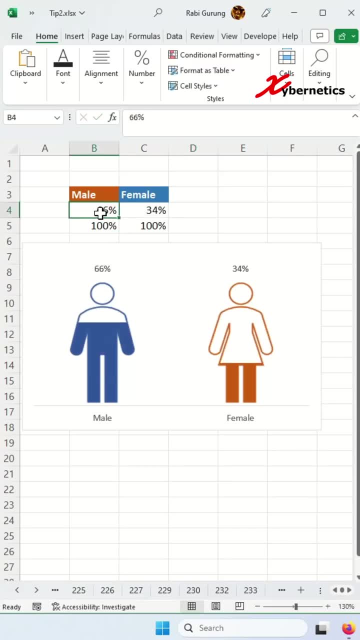 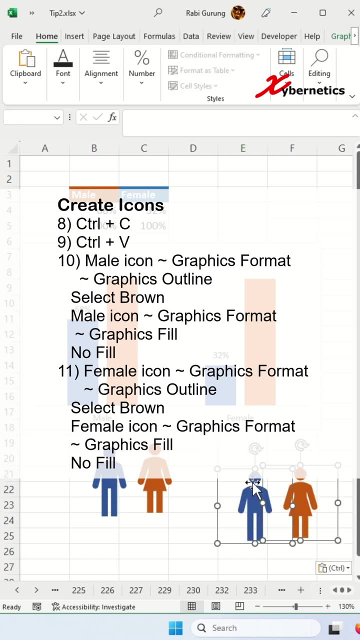 We're on a journey to create a male and female ratio chart that looks something like this. So let's continue. So we're going to select both of this again one more time and then press ctrl c and ctrl v to make a duplicate copy of it. Next, you're going to make a hollow out of this Select. 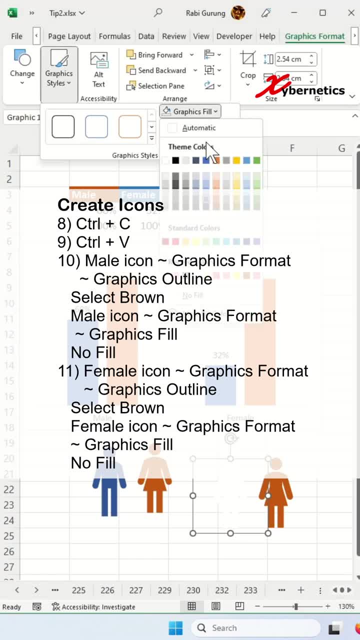 male icon. here Go graphic format, style and backfill. We're going to say no fill. and then we're going to say graphic outline: We're going to select the same blue color female. We're going to do the same thing. Select the female here. Go to graphic format, graphic style, graphic fill. We're 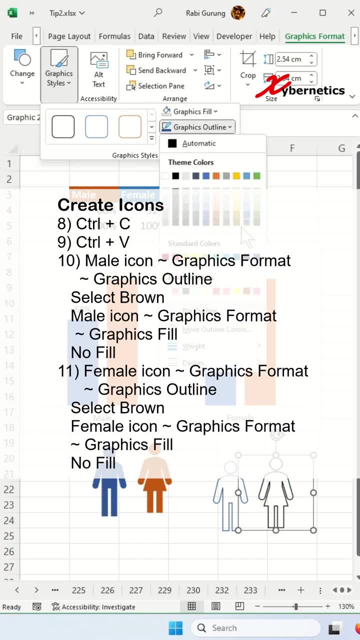 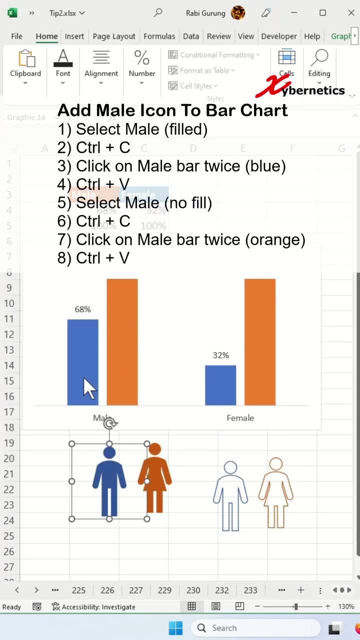 not going to say. we're going to say no fill, and then we're going to select outline as the orange color, The same color that we use just now. Next, we're going to introduce this icon to the bar chart here, Select the male ctrl c and then select this twice, like that. Make sure this is not. 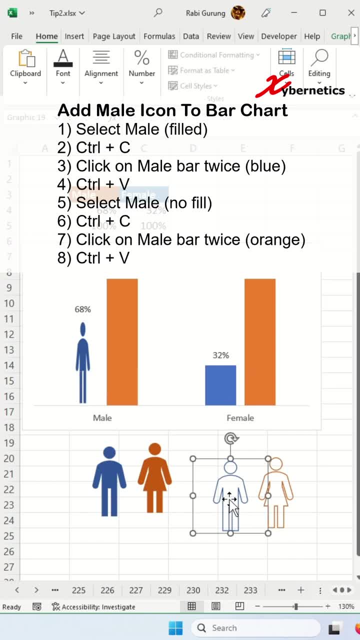 highlighted. Then you do ctrl v and then you select the male hollow, again ctrl c and then you select this one. here You see how this is selected. Click again one more time and the selection will disappear. and you press ctrl v here, Do the same thing with female. With that and we'll continue in.